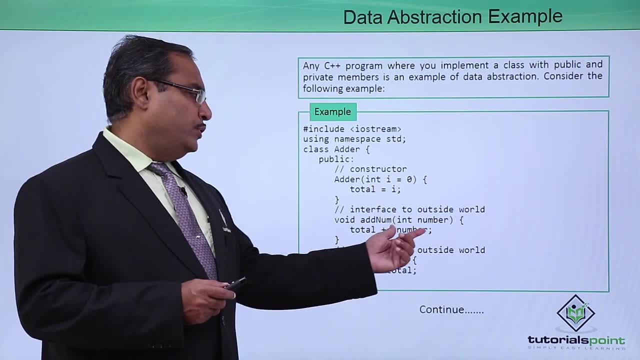 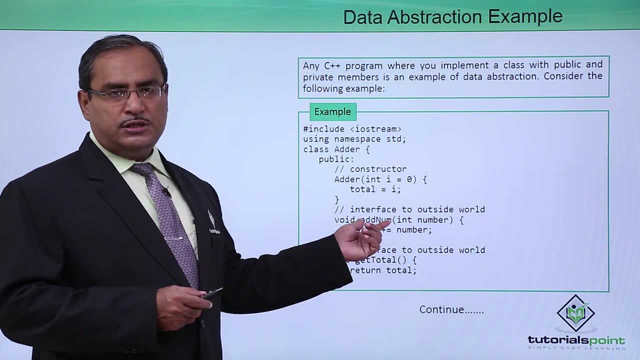 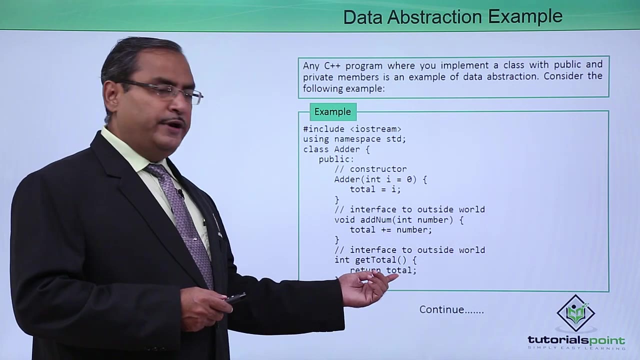 And now we are having another function, that is member function, that is ADD NUM, which is taking this number as input and which will add this number with the respective total and this ADD NUM. this function does not have any output argument. here We are going to get another function, that is the GET TOTAL, which returns the value of 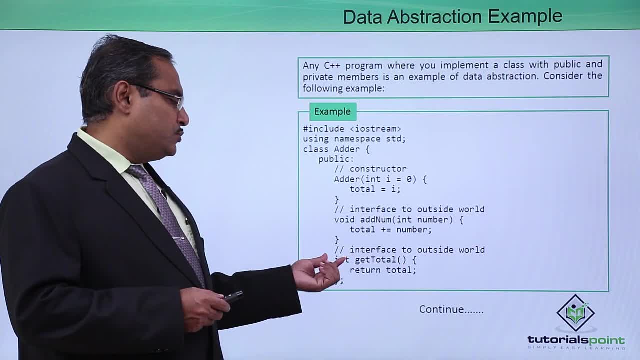 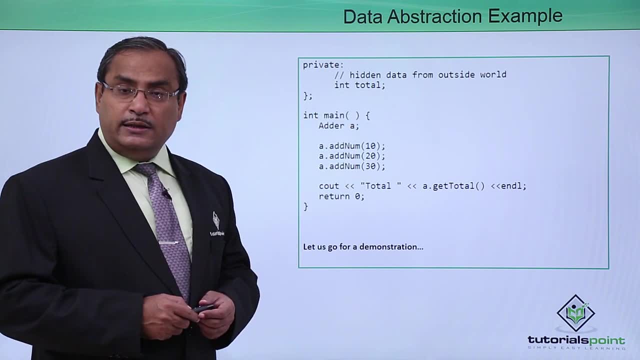 the total and total will be of integer type. So thats why the value has been return will be of type integer also. So here under the private section, we are writing this total. So as this total has been written under the private section, 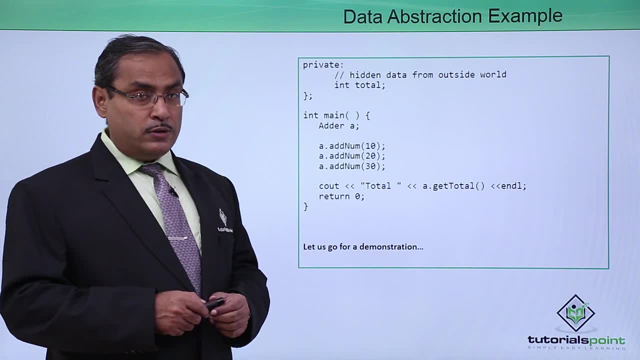 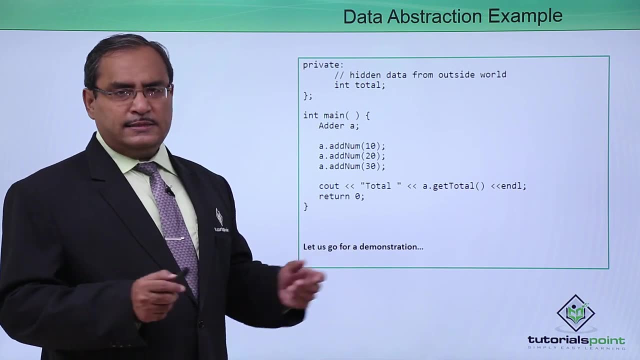 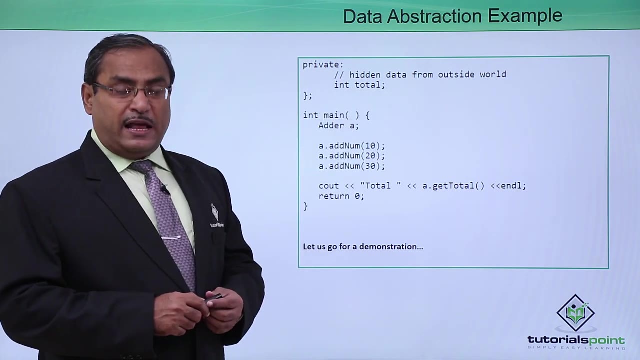 so it is not accessible from the global world, from the outside of this class. So all the member functions which are defined in this respective class can access this total. So there is no boundary conditions are there, but as it is defined under the private section, 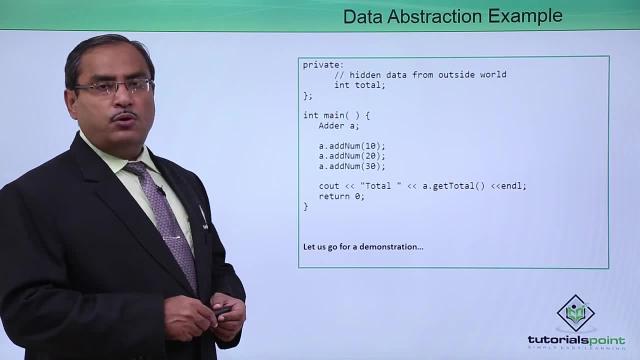 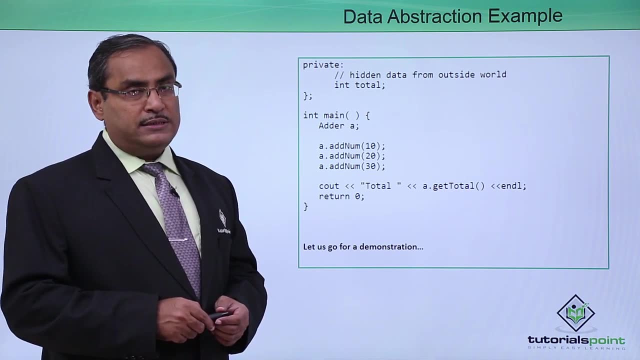 so hidden data from the outside world. So now let us go for object declaration of this class adder. We know that object is nothing but instance of a class. Whenever you are talking about some instantiation or instance, that means some memory spaces in the primary. 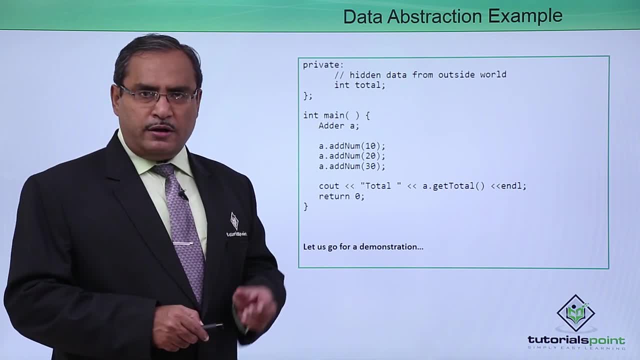 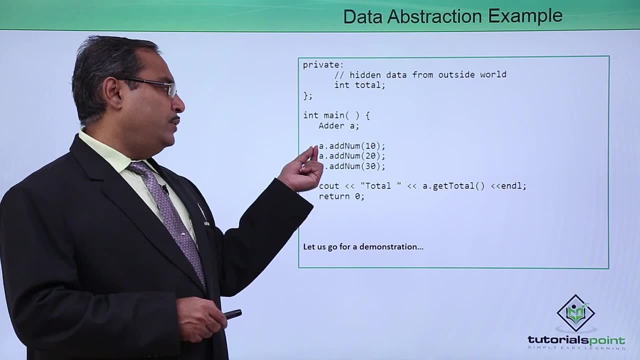 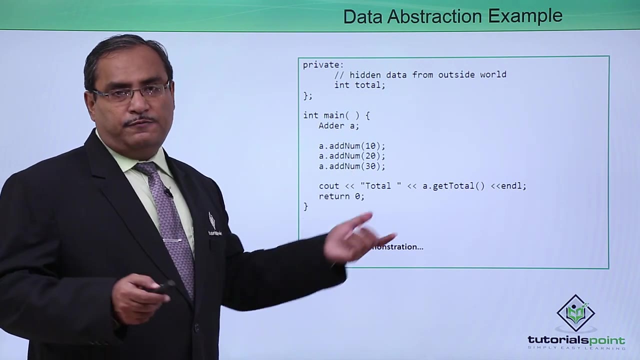 memory in the RAM of the system is getting allocated for that respective variable. So adder is the name of the class, a is the respective object. So a dot add name, a dot add name, rather, a dot add name, a dot add name. in this way I have called it for three times. 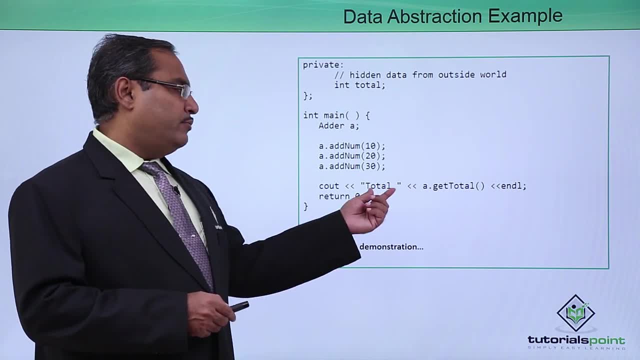 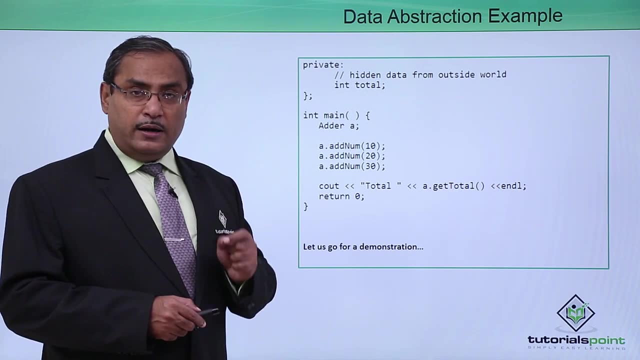 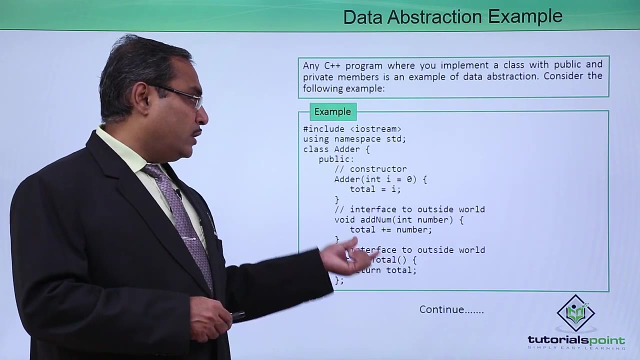 passing 10,, 20 and 30, and then we are trying to get the value of total to get printed, but as total is a member variable under the private section, so total cannot be accessed. To access total I must be using the function get total, which is under the section public. 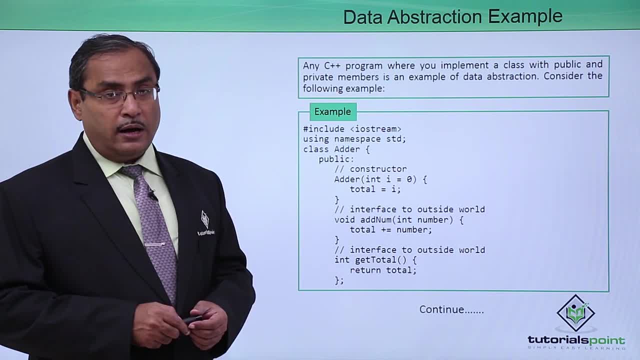 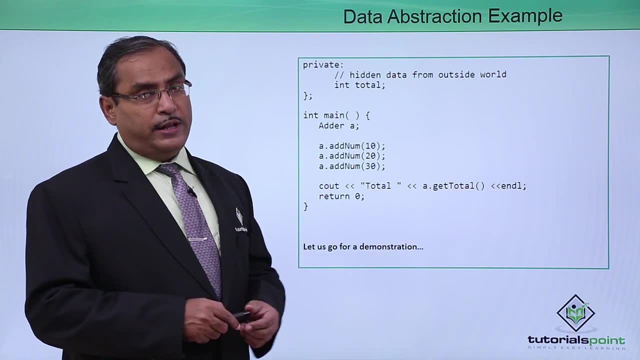 and that get total can access total. So that is not accessible. So the problem is that multiple users may not get a got total in the set of function and that get total does not make a problem for us. So as a result of that, we will be. 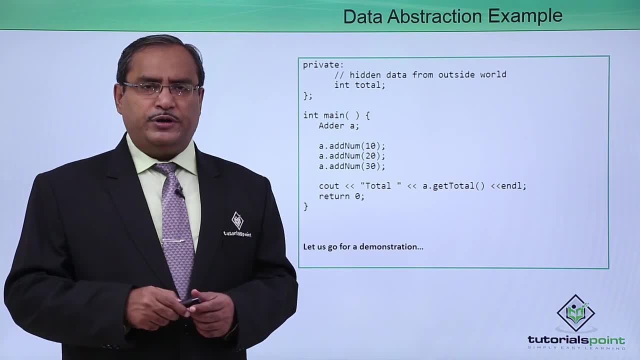 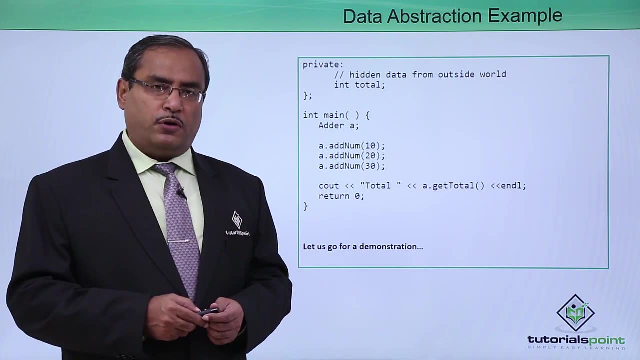 calling this respective function, that is, a dot, get total to print the value of the total. accordingly, I think it will be better if you go for one practical demonstration where we will be demonstrating that how this concept has been implemented in this code. So here, 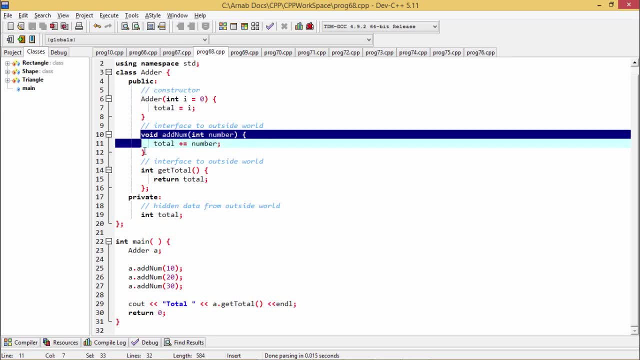 is the demonstration for you. another member function which is defined under the public section, so it is accessible from the outside world, and name of the function. member function is addNum, which takes a number as input argument and which adds this number with the total. there is another function which is defined under the public scope. 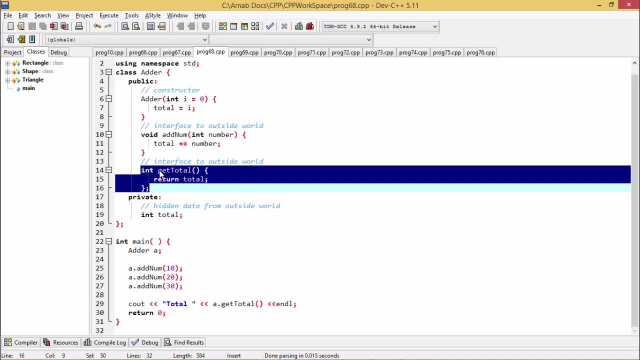 so it can be accessed from the outside world, and the name of the function is getTotal, which returns the value in total. so that's why this getTotal is having the output argument that is int. so here we are having this private section is there which is containing, which is having only one member function. 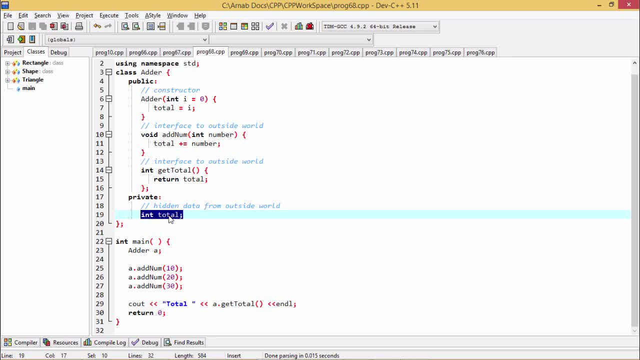 which is intTotal, and it is. it will remain hidden from the outside world because this total is defined under the private scope. now you see here, this total can be accessed from the public function and the name of the function from any member function defined under the same class, so a member function.